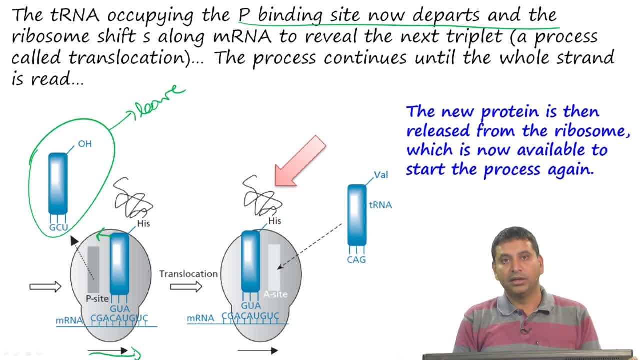 you have the mRNA moving in one direction and this process, wherein it moves or shifts and reveals the next triplet code, is called translocation. So this is a very critical component of protein synthesis because once the new protein is formed, it will be shifted out when the final- you know when the stop codon shows up. but 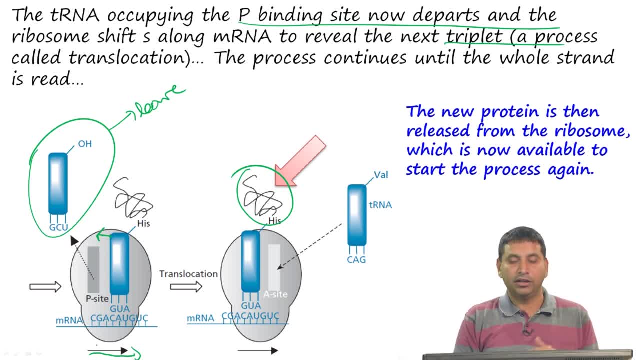 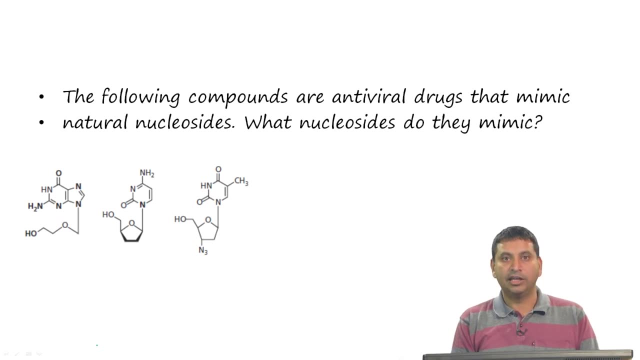 until then, you need this process to happen in a very smooth manner and the translocation is an important part of this entire process. The next question: the following compounds are antiviral drugs and they mimic the natural nucleosides. So, as shown over here, what nucleosides do they mimic? So here is we look at in detail. 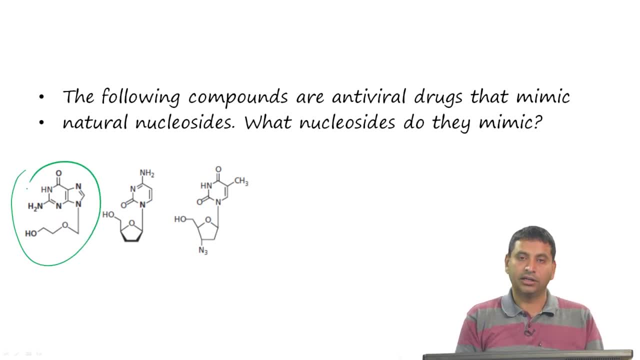 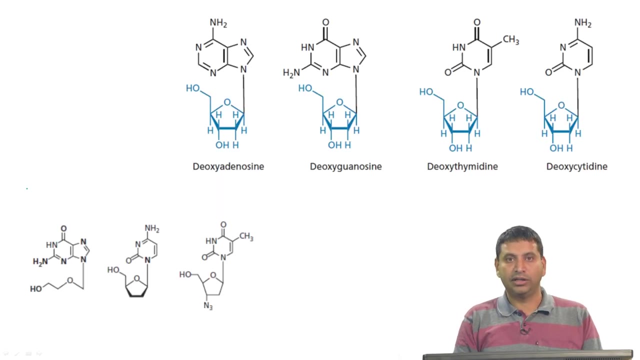 some of these examples of how these drugs work In the later part of the course, but let us. the question here is asking us to understand which nucleosides that they they mimic. So, in order to answer this question, let us first draw out the natural nucleosides that are present, and so we see here that this is the 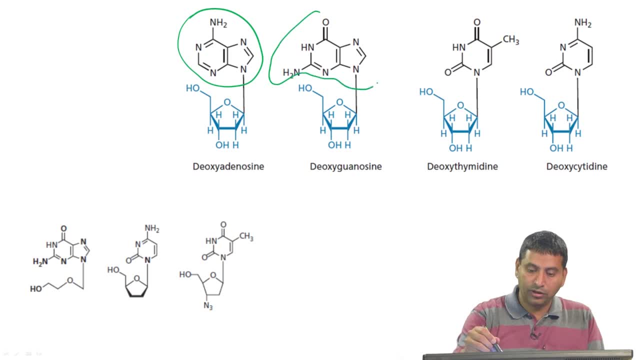 structure of adenine, this is the structure of guanine, this is the structure of thymine and this is the structure of cytidine. So let us start with the first example. So here this compound to me looks like guanine. So this mimics guanine, as shown here, and this: 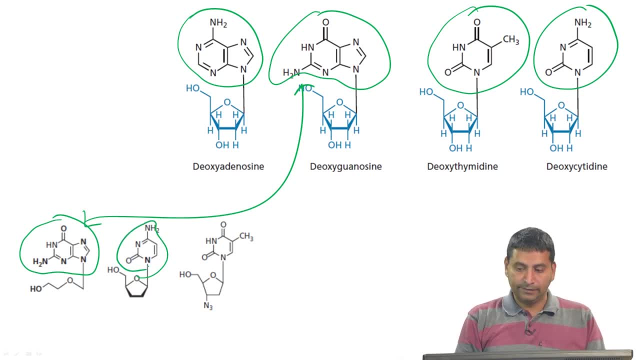 compound here is has a cytidine like molecule. So here is the how we would match this. and the last compound is mimicking thymine. So what we would expect with these antiviral molecules is that, since they have an identical structure to the base, then the hydrogen bonding. 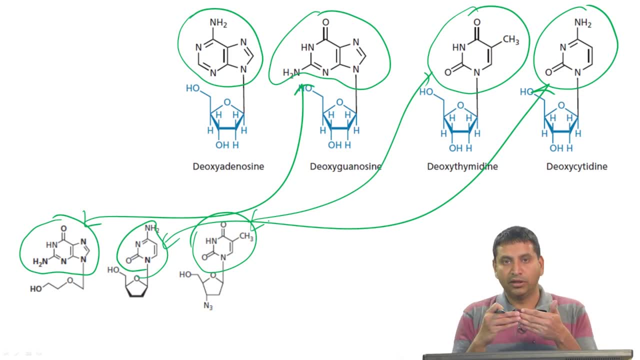 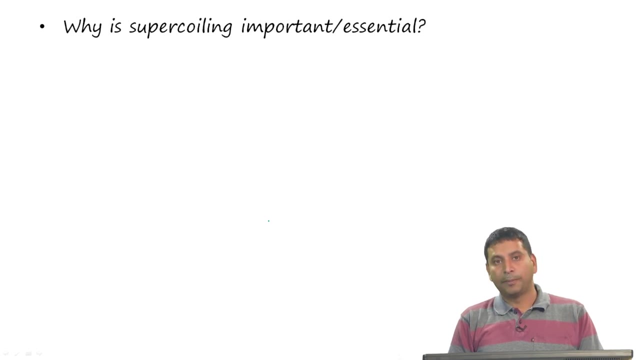 that would occur between the complementary bases would be similar, So antiviral drugs act in this manner. We will look at this in more detail towards the later part of the course. Why is supercoiling important or essential? So DNA supercoiling is a is very important. 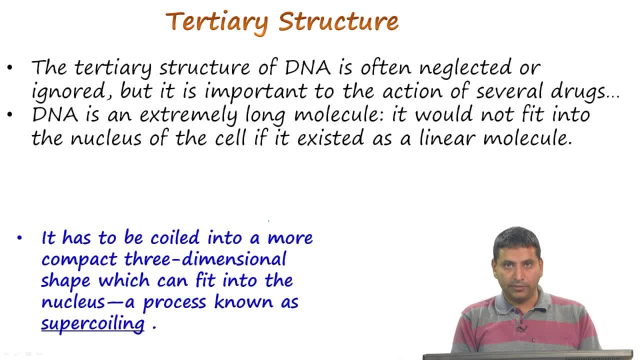 because it helps with the tertiary structure of DNA. Now its DNA is extremely long molecule and it would not fit in the nucleus of the cell if it existed as a linear molecule. So if you take DNA to be a linear molecule, it is extremely long. So what happens is that it 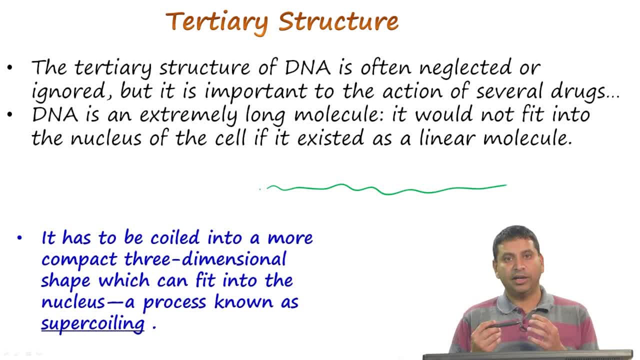 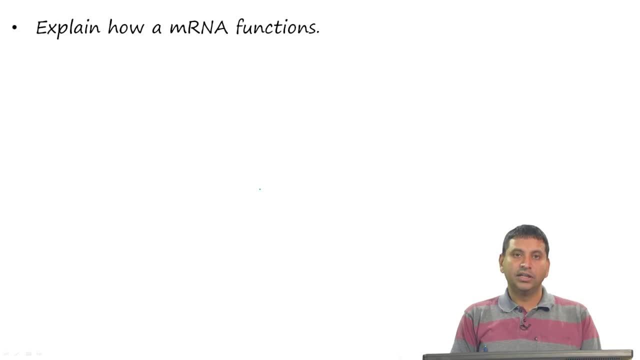 is coiled into a more compact three-dimensional shape which can fit into the nucleus, and this is process is known as supercoiling. So therefore, supercoiling is very important to be able to fit the genetic material in the nucleus. Next question is explain how mRNA functions. So mRNA, as we know, is basically messenger. 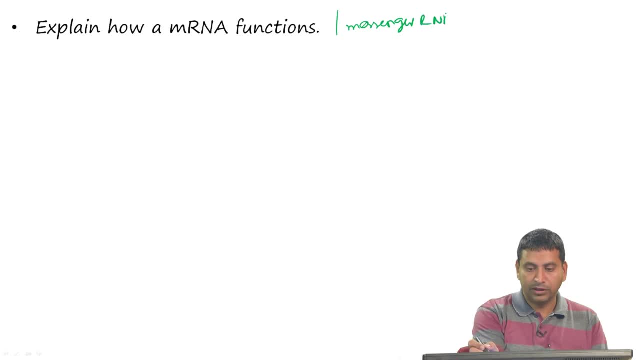 RNA and in order to understand what messenger RNA is. messenger RNA takes a message from DNA to the protein synthesis machinery, So this process is called as transcription- Transcription. what does it do, Transcription? what is a transcribed DNA? It is called transcribed. 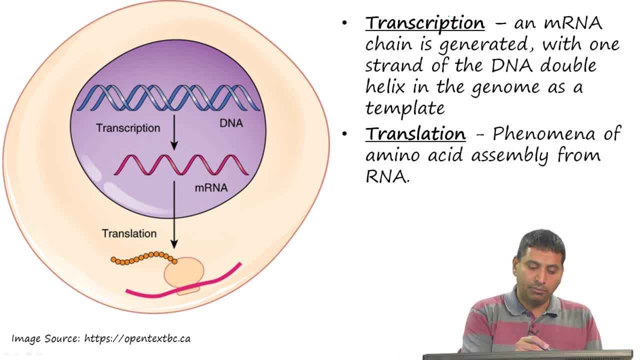 gene. So what happens is that it takes a message from this gene and it puts it into the protein, is a process by which a mRNA is produced using the code from DNA, and this allows us to transfer the information in DNA and send it to the ribosome or endoplasmic reticulum, where the 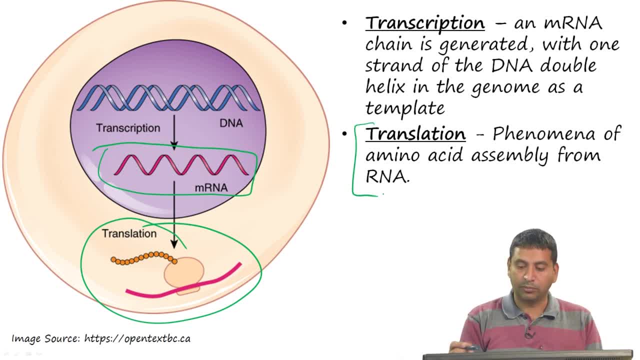 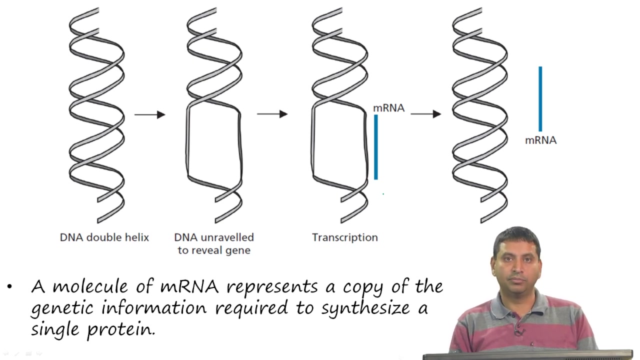 protein synthesis is occurring. So protein synthesis is the process is called translation, where this code that mRNA is carrying with it goes to the endoplasmic reticulum and the ribosome there and that is converted using the machinery to produce a protein. So mRNA works. the transcription happens first by exposing the gene and then the mRNA is. 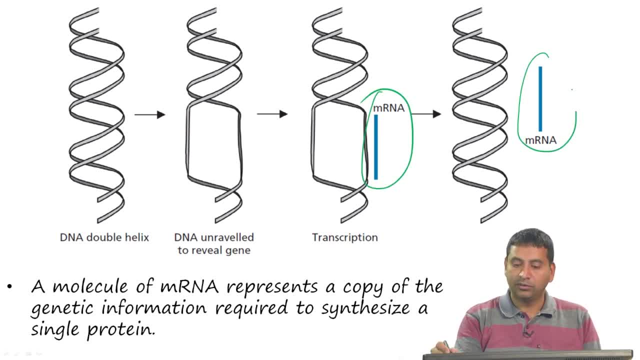 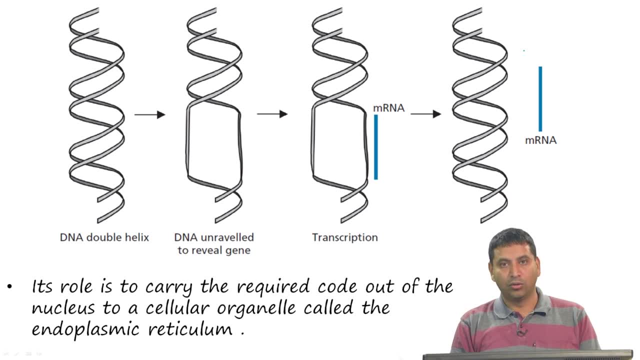 synthesized over here and then mRNA is produced. So its role, as we discussed earlier, is to carry the required code. So what is the function of the protein? The function of the protein is to carry the required code to the endoplasmic reticulum. 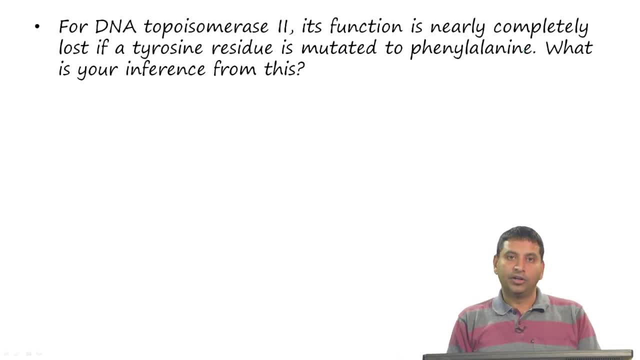 out of the nucleus to a cellular organelle known as endoplasmic reticulum For DNA topoisomerase II. its function is nearly completely lost if a tyrosine residue is mutated to a phenylalanine. What is your inference from this? 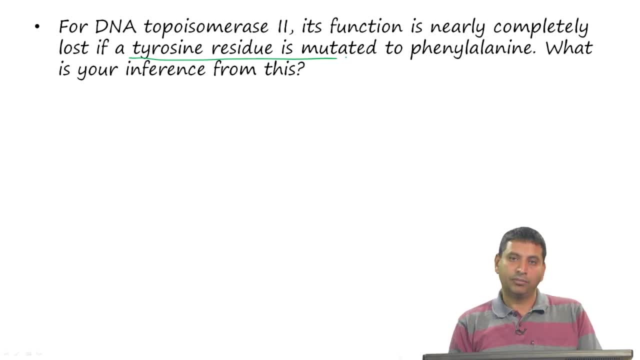 So, again, going along what we have looked at in the previous classes, the way in which we would understand the function of a protein, in this case DNA topoisomerase II, would be to carry the protein. It would carry out what is known as a side-directed mutagenesis. and this side-directed mutagenesis 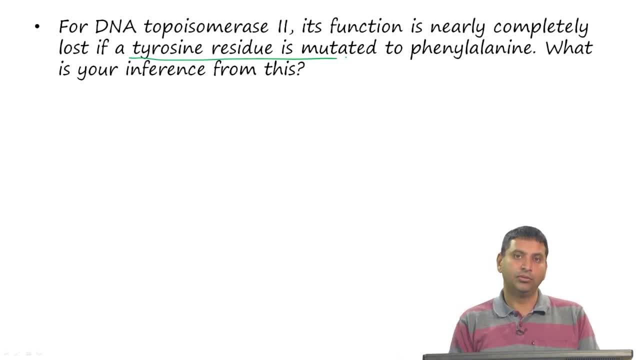 basically replaces a protein, an amino acid residue, with another amino acid residue. So if the tyrosine here is replaced with a phenylalanine, then the activity of DNA topoisomerase II is almost completely lost. So therefore the tyrosine residue must be a very important part of DNA topoisomerase. 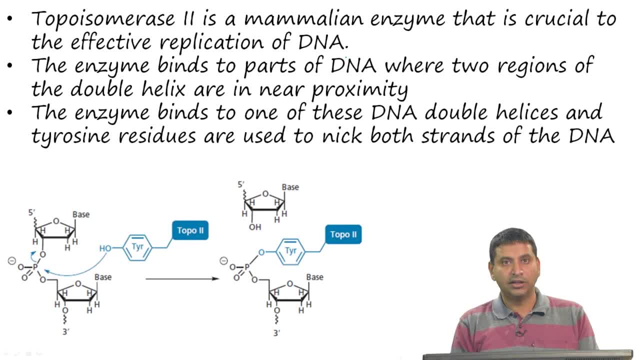 II activity. So we already have learnt in class that topoisomerase II is a protein. Topoisomerase II is a mammalian enzyme that is crucial for effective replication of DNA. So this enzyme binds to parts of DNA where two regions of the double helix are in near 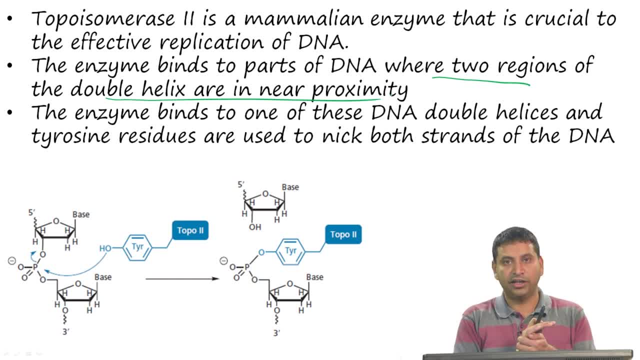 proximity. Then the enzyme binds to one of these DNA double helices and the tyrosine residues are used to nick both the strands of DNA right. So this tyrosine residue over here. what it does is it reacts with this phosphate diastole. 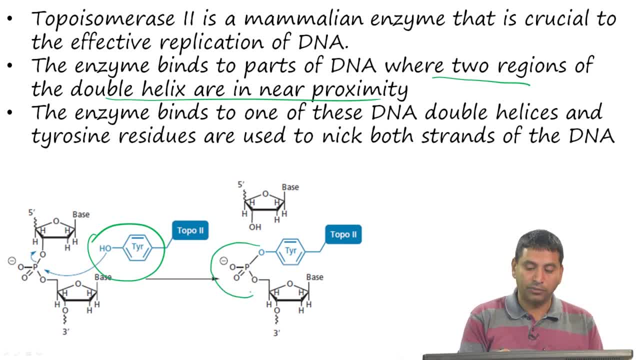 bond here and produces a nick. Because you now have a double helix, The separation of the single strand to there is a nick that is produced. So therefore, if you now mutate, this tyrosine residue, which is this hydroxyl group, is: 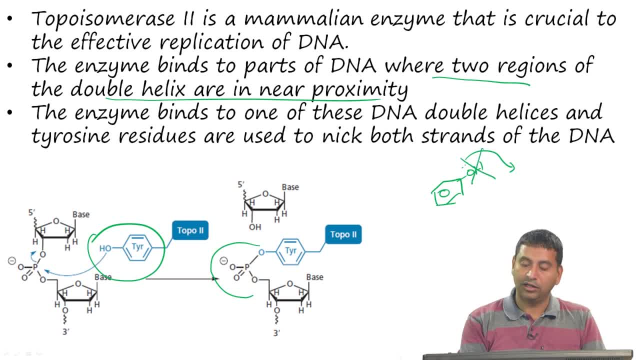 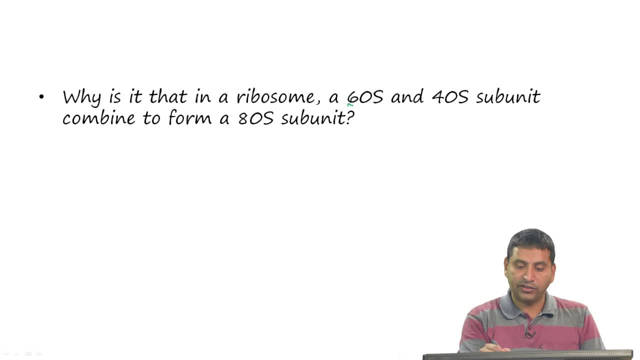 very crucial. if you remove this and only use phenylalanine, then there is no possibility of this reaction occurring and therefore the enzyme loses its activity. The next question is: why is it that in a ribosome, A 60S subunit and a 40S subunit combine to form a 80S subunit? 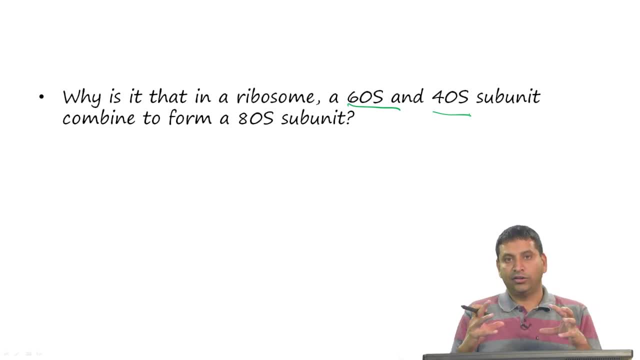 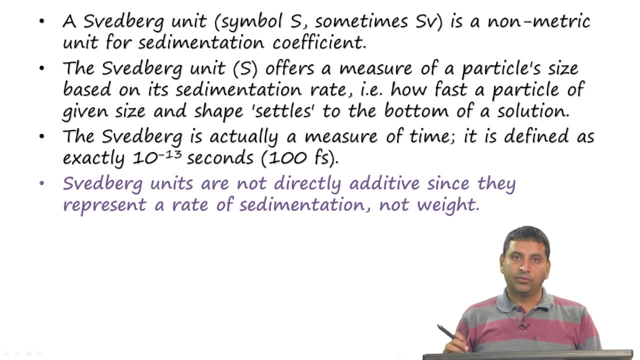 That means if I combine a 60 and a 40S, I should get a 100S, but I actually get 80S. So the answer to this is that the S stands for Svedberg. So Svedberg unit is a nonmetric unit, which is known as a sedimentation coefficient. okay, 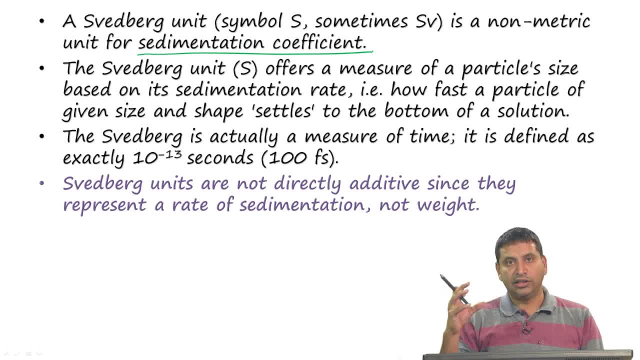 So Svedberg offers a measure of a particle size based on the sedimentation. So Svedberg unit is a nonmetric unit which is known as a sedimentation coefficient. okay, It is based on the sedimentation rate, that is, how fast a particle of a given size and